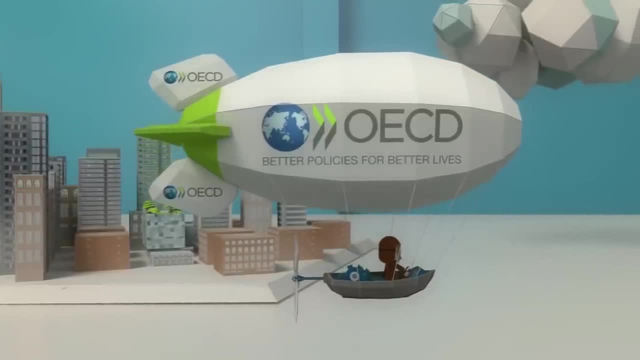 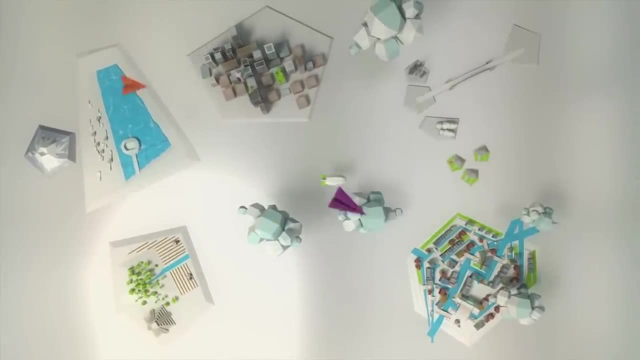 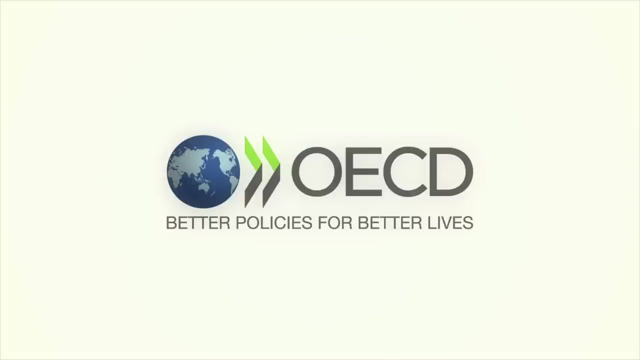 The OECD supports countries' preparations for climate change by bringing public and private actors together, providing analysis and policy advice for adaptation. Working together, we aim to support smart action to tackle climate change. For more UN videos, visit wwwunorg. 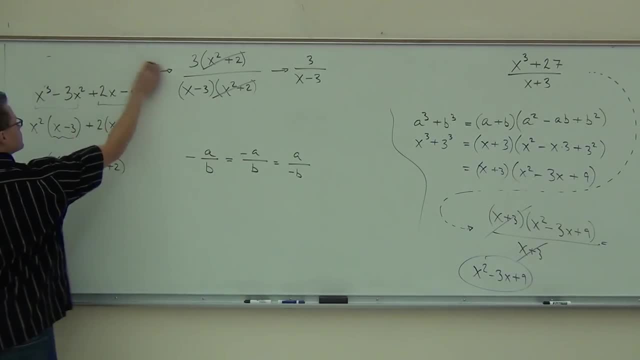 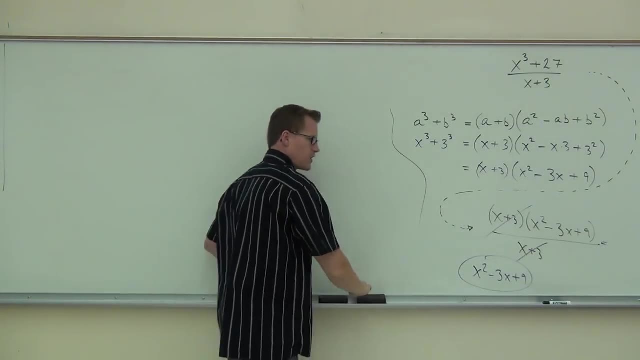 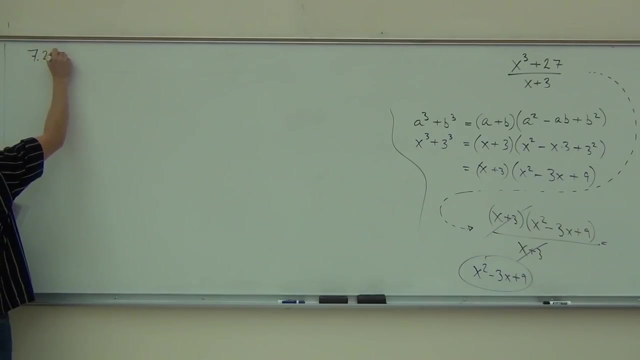 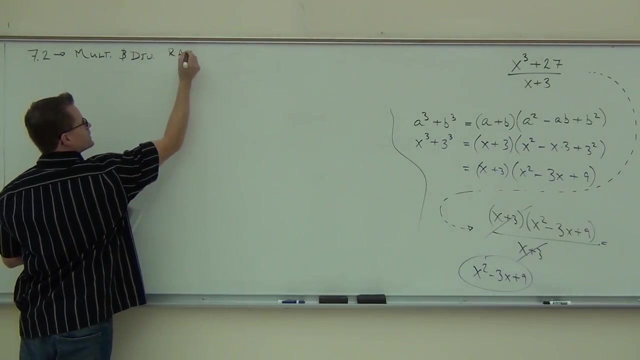 So we're going to go on to section 7.2.. For the rest of our time, we'll talk about how to multiply and divide rational expressions. That just means fractions of polynomials, just like we've been dealing with Multiplying and dividing rational expressions. 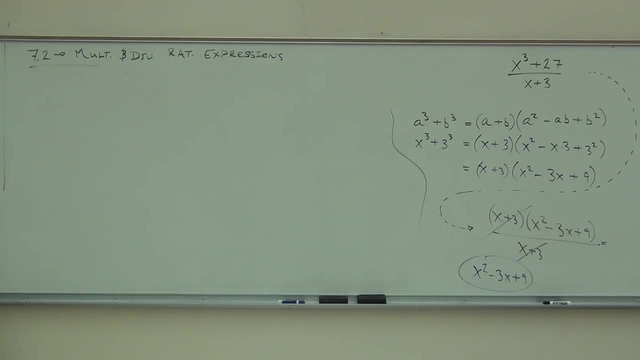 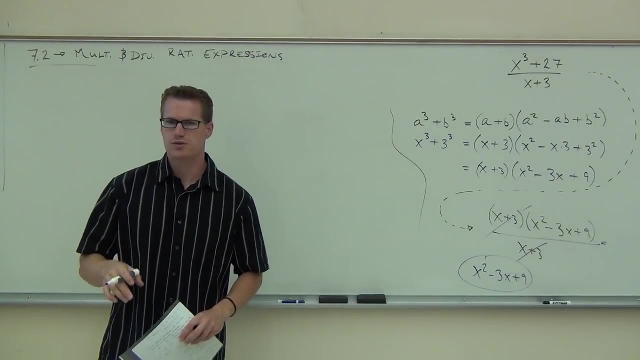 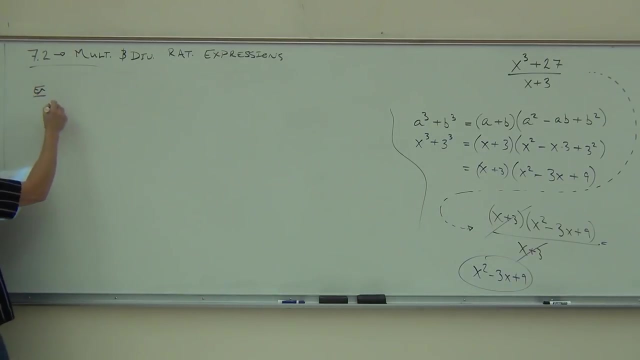 Multiplying, dividing rational expressions, Very, very, very much like working with fractions. With fractions, you really have two options, right? Here's your two options for multiplying. If I just give you some regular old fractions, we can do something like that. 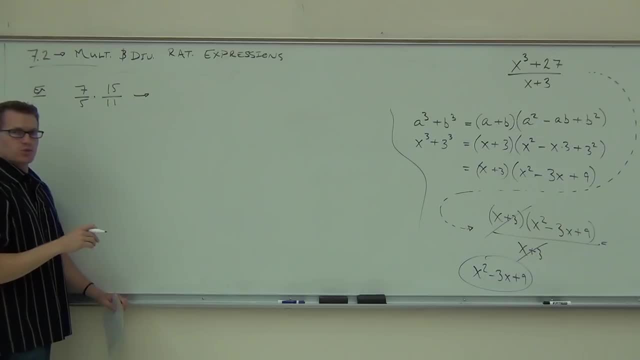 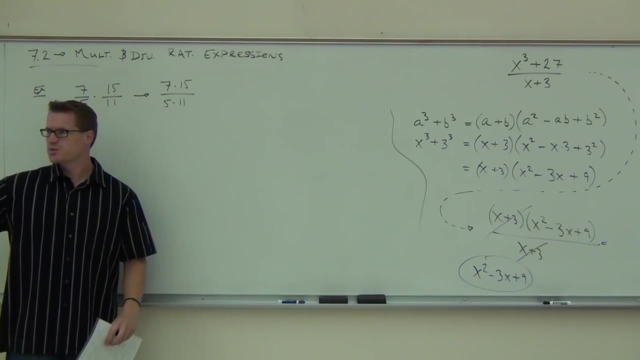 And you have two options really. You could go and multiply the numerators, couldn't you Do like 7 times 15,, 5 times 11.? Because we know when we multiply fractions we just go straight across. Do you recall that from a long time ago? 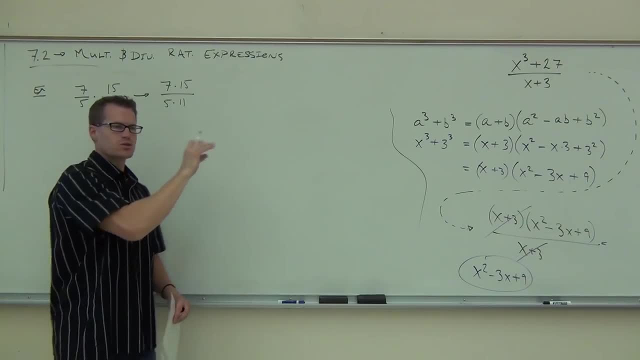 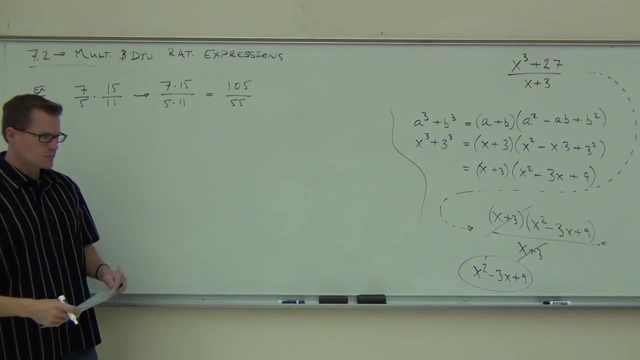 I hope so. I hope you do right. We just go straight across And we get something like 105 over 55. And then you'd have to simplify, wouldn't you, if you did it this way. But there's really another option. 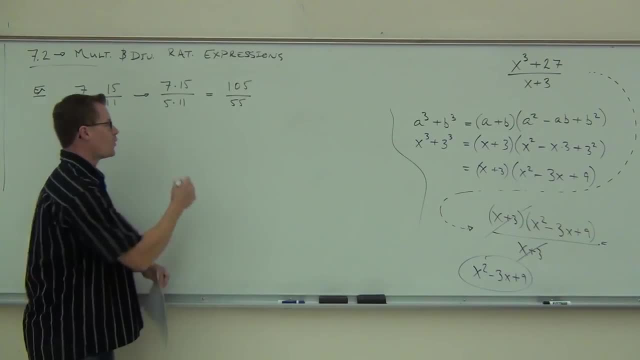 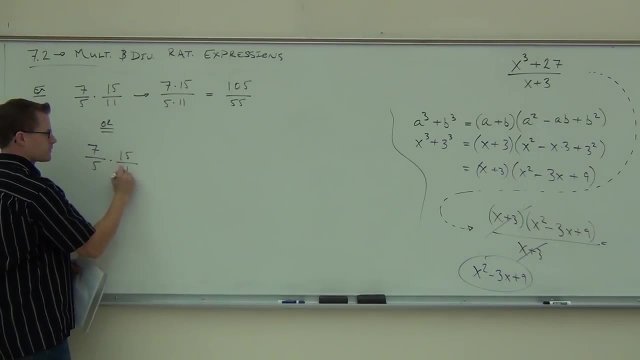 And this is probably what you prefer to do when you multiply fractions. So the, or What we're going to do, when you get down to this part of it, you still have to write it as 7 times 15 over 5 times 11..